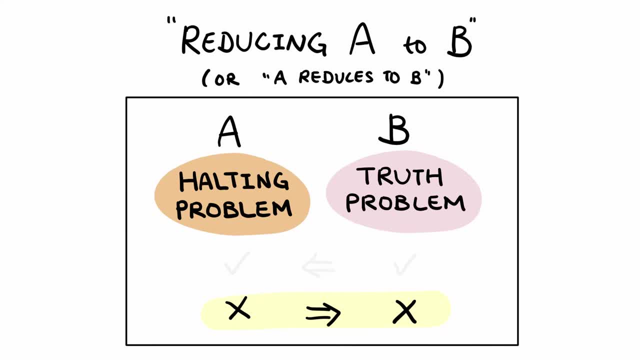 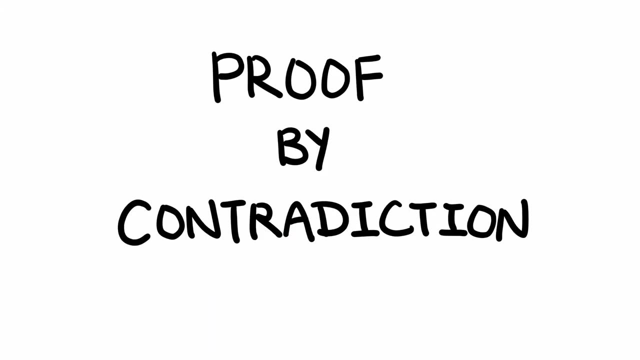 problem is undecidable And all that was left to cover was to show that we can perform the reduction, which is what we will go through in this video. To show that a problem is undecidable using reductions, we do it through a proof by contradiction. I've included the proof in writing. 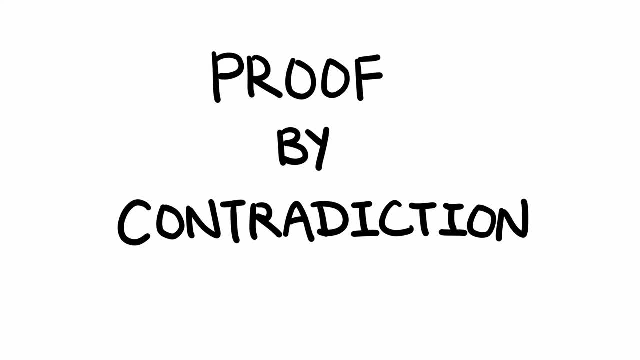 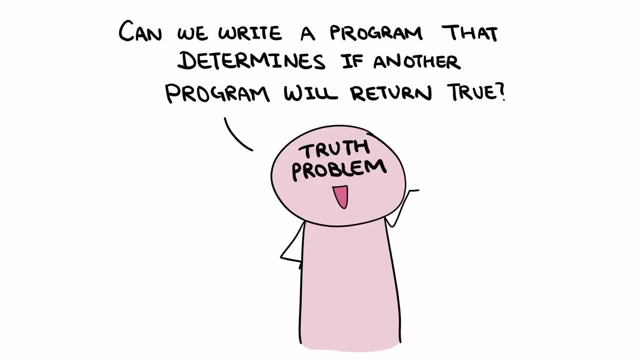 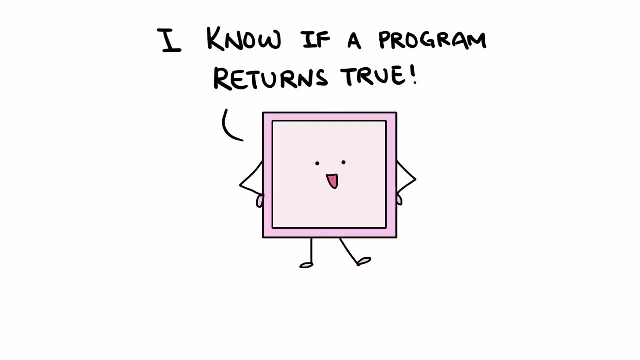 in the description below as a reference, so feel free to look at that to follow along. The truth problem asks whether we can write a program that determines if another program will return. true, Let us now assume, for the sake of contradiction, that there is a program that 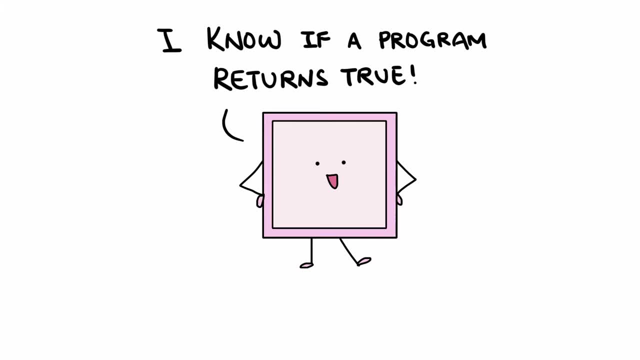 decides the truth problem. We now show the reduction. So this new program- let's call it t- will take a program as input and return true if a program returns true or return false. if the program does not return true, And when it does not return true, it may either be because the program 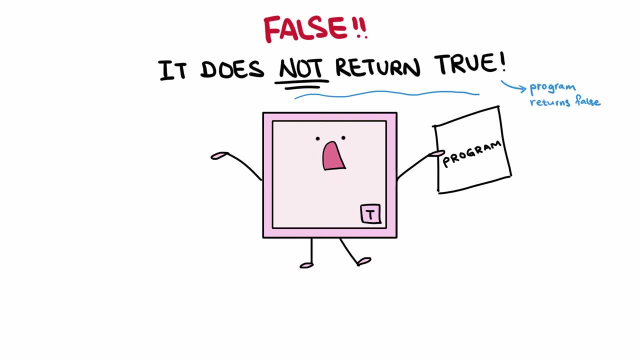 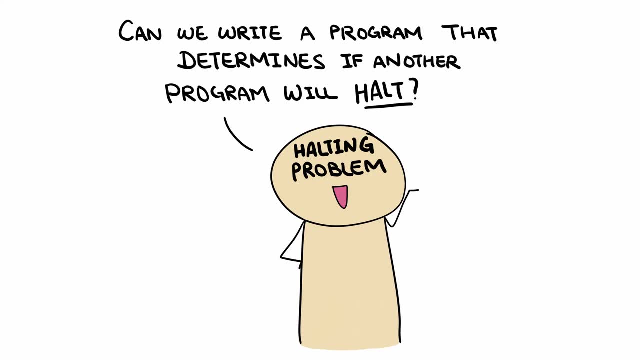 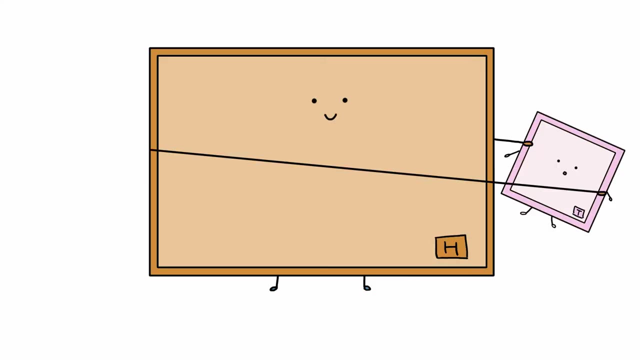 returned false or the program simply didn't return true. So let's take a look at this new program, In case you forgot. the halting problem asks whether we can write a program that determines if another program halts. Now we build a program, which we call h, that uses program t to solve the 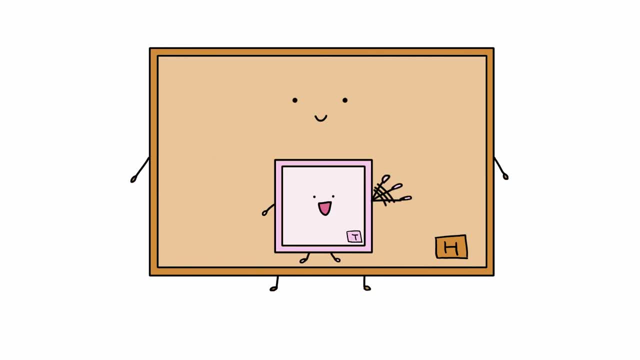 halting problem. We know this actually cannot be done, but we assume it can be for the sake of contradiction, because we want to show that we can reduce the halting problem to the truth problem. So how can we build h using t? We define h as follows: h takes in a program as input. 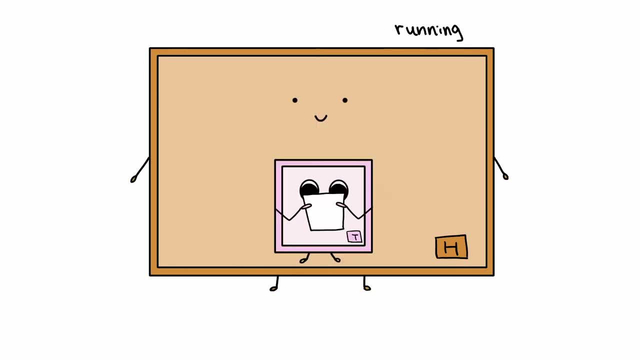 and immediately gives it to t. t then scans through the program and tells us if the program will return true or if the program does not return true. At this point we know that if the program returns true, the program most certainly halted and h will return true. 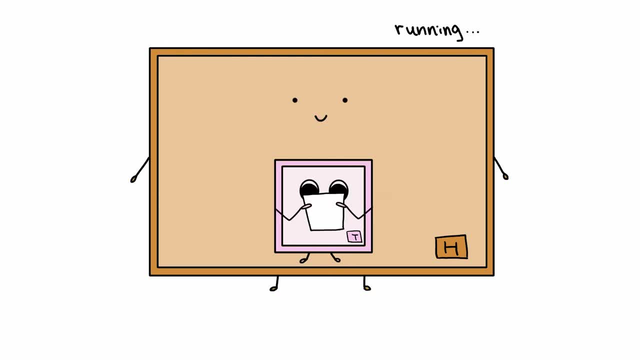 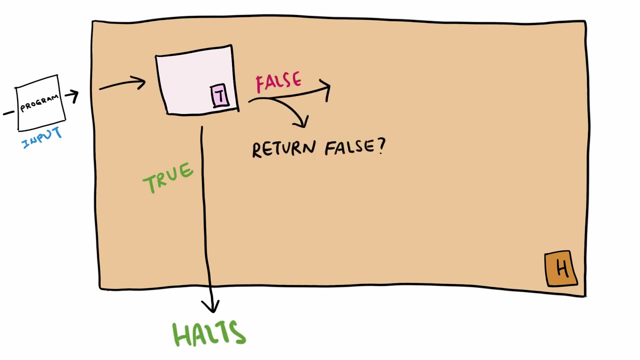 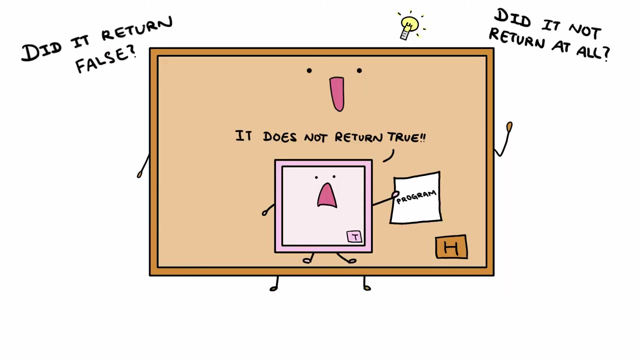 However, if t determines that the program does not return true, then the program either returned false or it may have just never stopped running. But to properly define h and show the reduction we need a clear description for when h returns false. So to do that we may have to get a little creative. If t said that the program did not return true,